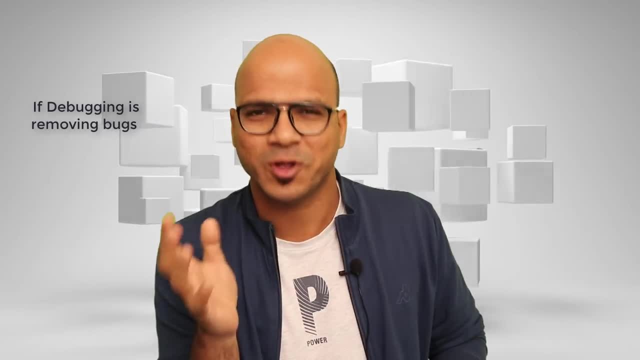 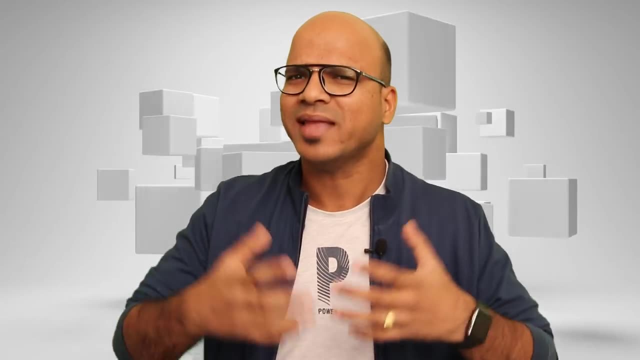 right. What about coding then? If debugging is removing bugs, then coding is actually adding bugs, right? So every time you code, you add new bugs. Now, even if you don't do it intentionally, it happens, you know, because we are trying to do it intentionally, right? 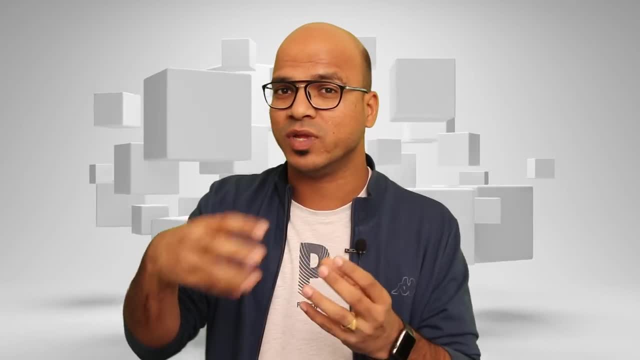 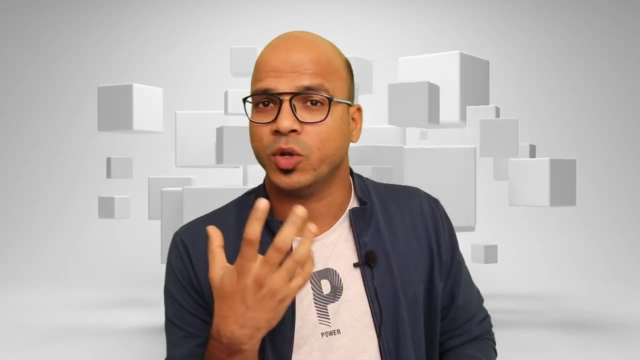 We are trying to solve a problem And around that, you will be writing some code which will increase bugs. Okay, now, how do you manage this stuff? right, Because if you increase bugs, of course at some point you need to read your own code. you need to understand. 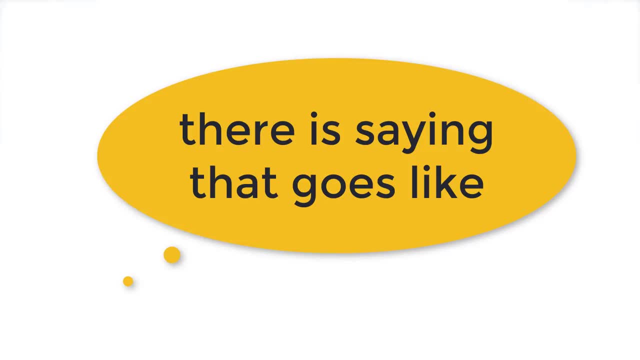 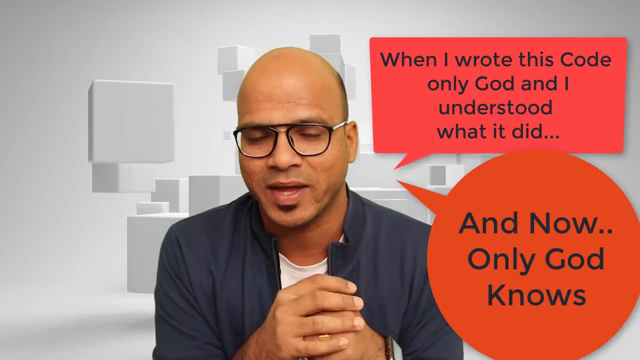 how to remove those bugs, and your software should be maintainable. When I wrote this code, only God and I understood what I did, And now only God knows right. So it happens. you know, when you write a code, after some time even you will not understand what you. 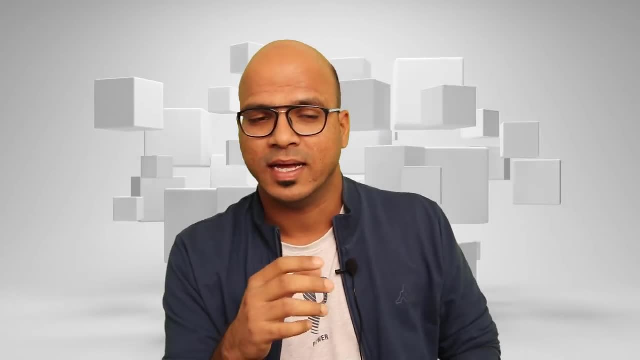 have written, Because when you have thousand lines of code it is difficult to translate right. So when you write a code, after some time even you will not understand what you have written. Take note, remember. The second problem is if you write everything. 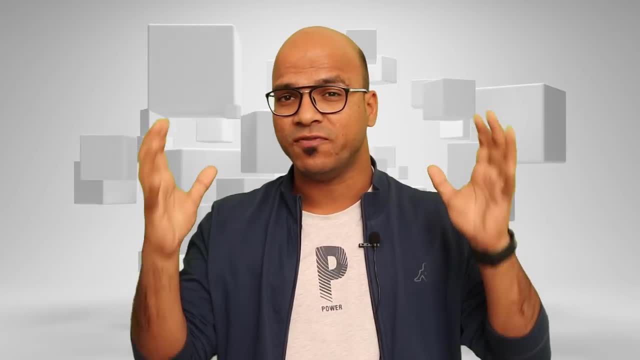 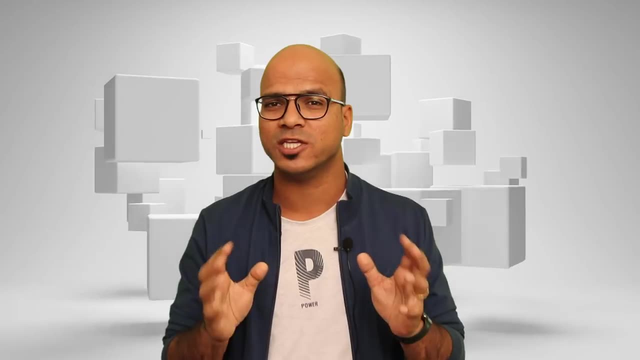 on the same page, or if everything is at the same place, it is difficult to manage it, And if you change one point, it may affect other code as well, And that's where what you will do is, if you want to solve this problem, we will be using our concept of modules. 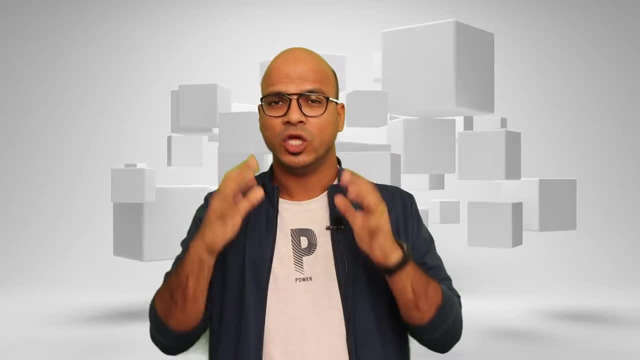 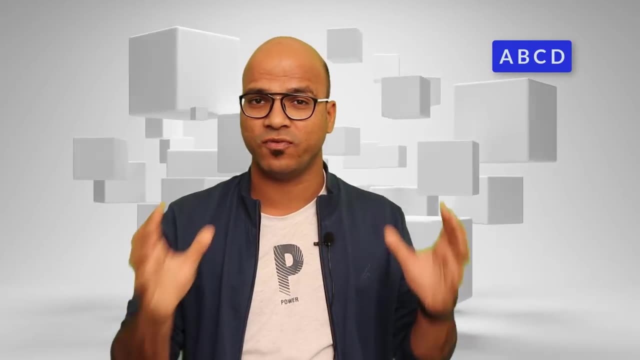 So instead of writing one big software in one file, you will break it down into small, small parts, right? For example, let's say, if you have ABCD as a software, you want to build a software in which you have these four features, and that is one project, right? 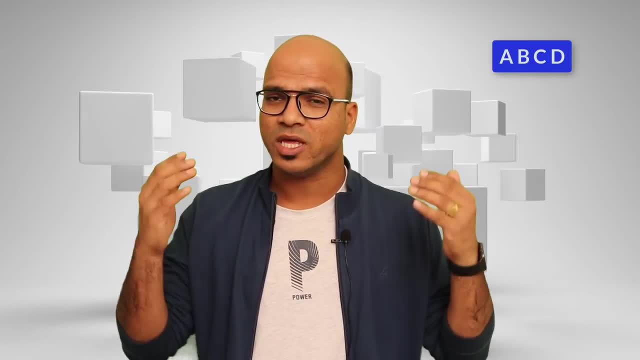 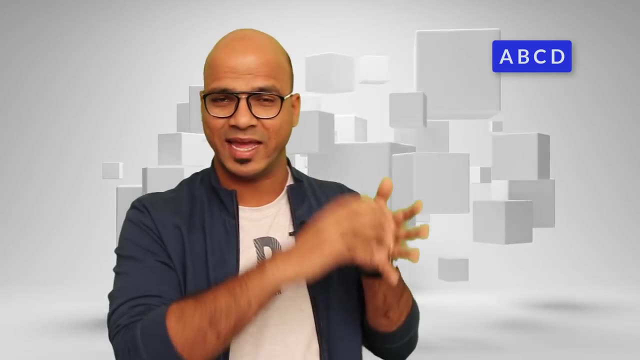 It is a combined project, Yes, Grab. so what you will do is before, even before starting the actual project, what you will do is you will break it down, the components on paper, so you will write: hey, we have abcd, now we have to break it. 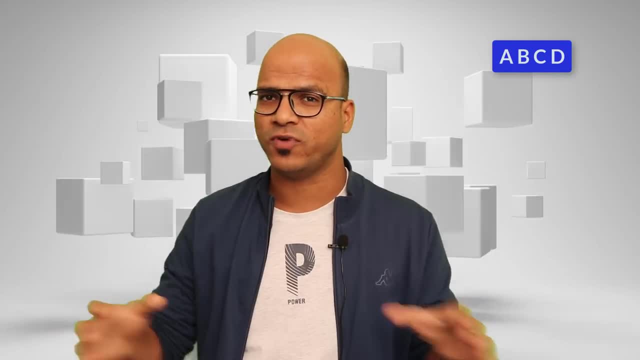 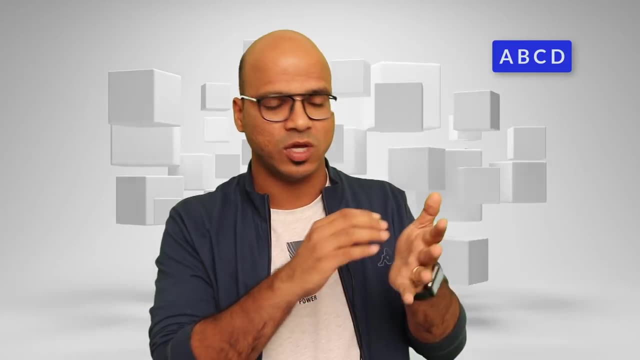 down in logical parts, right? of course you cannot simply break down software. you have to think about it. you have to break it down in logical parts, right? so all the same features should belong to same module. so you will say, okay, we have abcd. well, a and c can be one module and b and d can be. 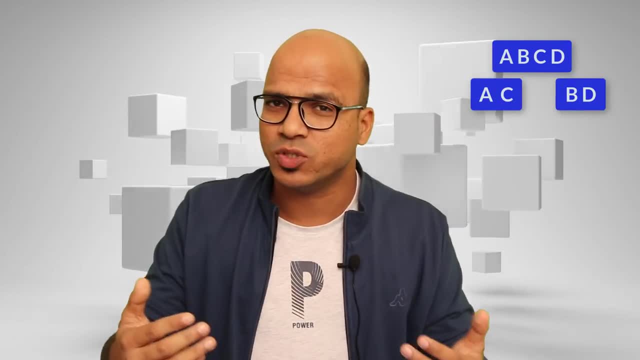 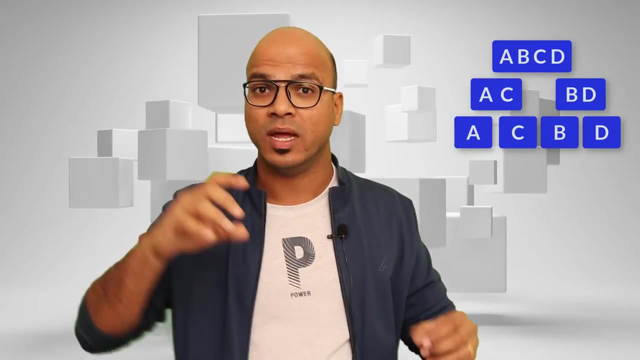 one module, okay, so that's what we have done. and then further you realize: okay, we can actually also break it down a and c. so you have saying a module, c module, b module and b module. so we are breaking things down. the advantage is you will be building four different modules, right? the first? 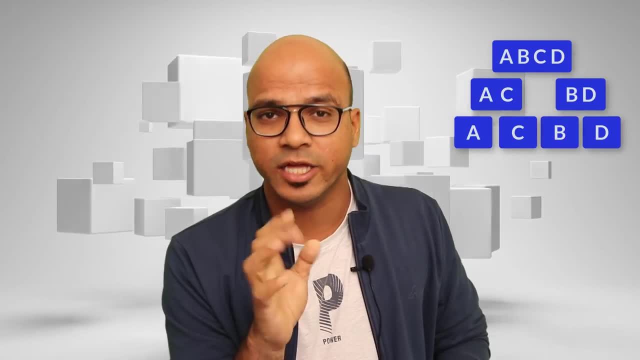 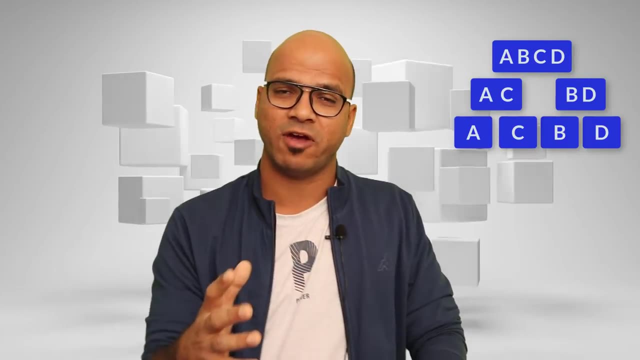 advantage would be: if you want to change something in a, it should. it will not affect other modules, right, because they are separate. now it may if you are doing some tight coupling stuff there, but normally it doesn't affect, so when you write a code. if you change something in a, it will not. 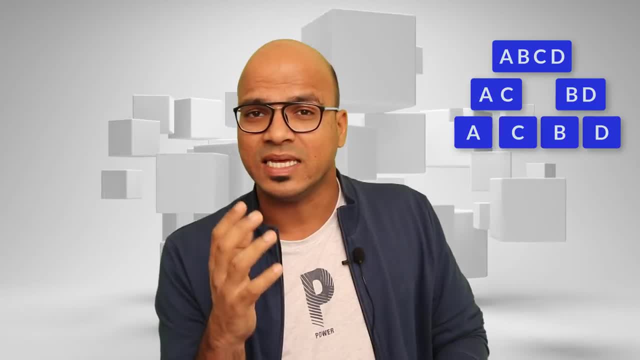 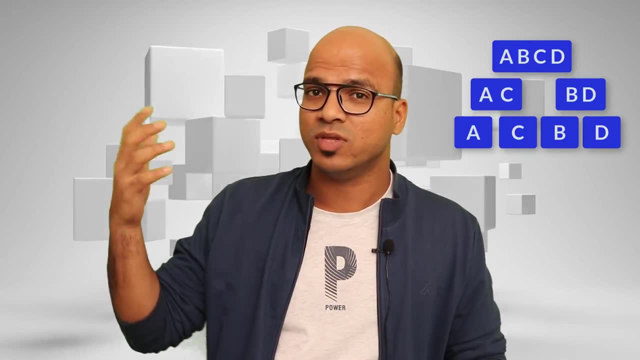 affect other modules, or it may not affect other modules, but it will not affect other modules, other modules. but the next thing is you can also reuse your modules. example: let's say, after this project, you are building a new project with the some similar features. example: now, this time you 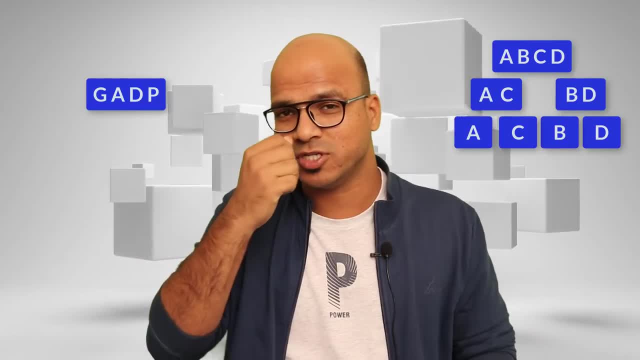 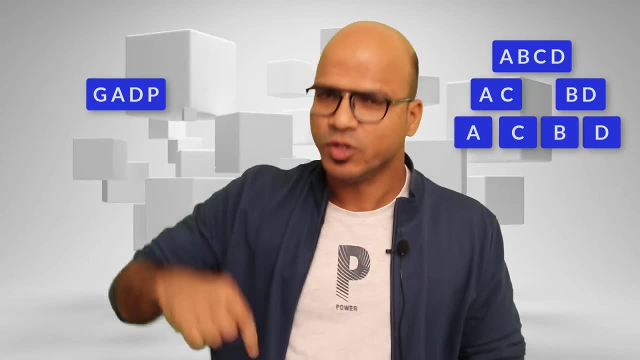 are building maybe g, a, d, p, so we have this other project now. here you can actually use a and d module because you have to build it right. so that's the advantage of using modules. now can we do that in a project? in fact, we'll not be building a complex project here, let's do it simply. but then 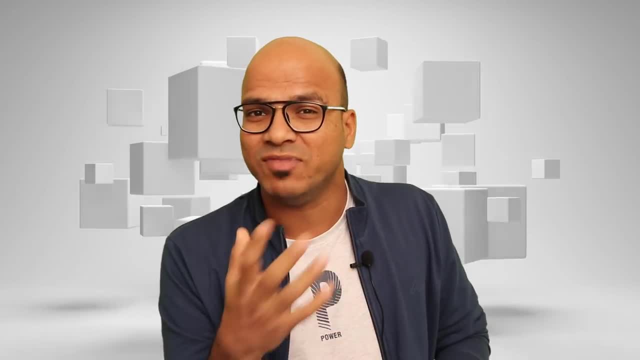 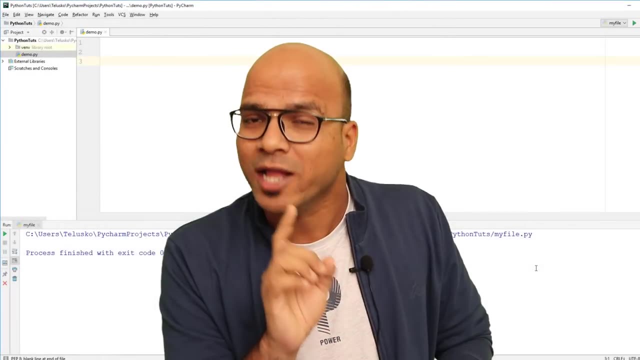 if we talk about a module, what it will have. so in python we have this concept of variables, we have functions, we have code, we have functions, we have functions. so that's the advantage of using modules: classes, right again, we'll be talking about classes later, but we have that concept, so in one. 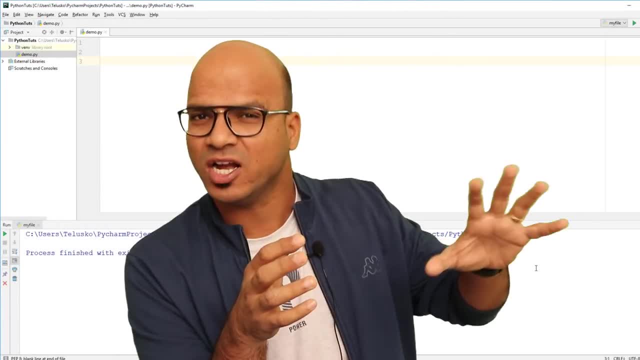 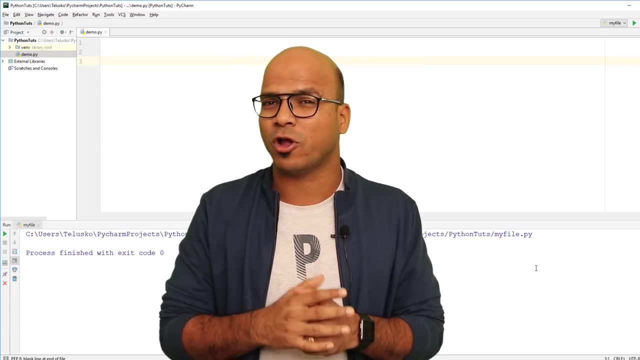 module. you can have all the different stuff, right. so we can have variables, we can have functions and we can have a class, or you can imagine, at this point your one module will be one file. so the way we are doing a file here, we have demopy. this is your one module, right, we can create another file. 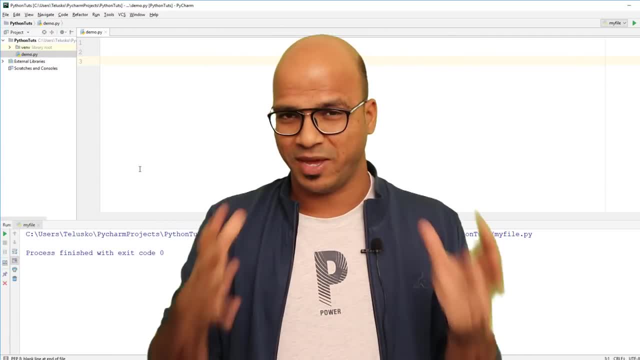 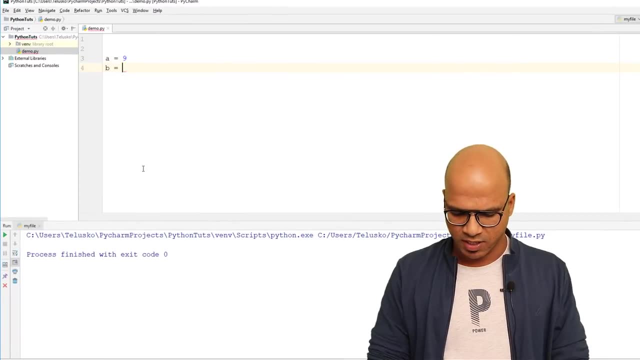 as a separate module. let me show you something. so let's say, this is my main file, right, and here i want to add two numbers. so what normally we do is we simply say a is equal to nine and you say b is equal to seven, and here you will add those two values, right? 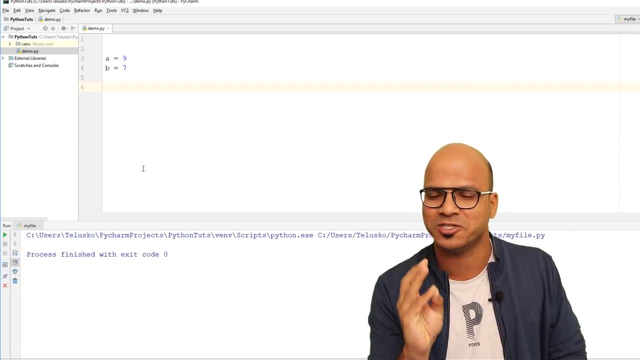 maybe you want to perform all the operations right- addition, subtraction, deletion, multiplication- so you can do that here itself. or you can create functions- and now we know how to create functions right, so we can do that here. but we can create modules right, so you can create those four. 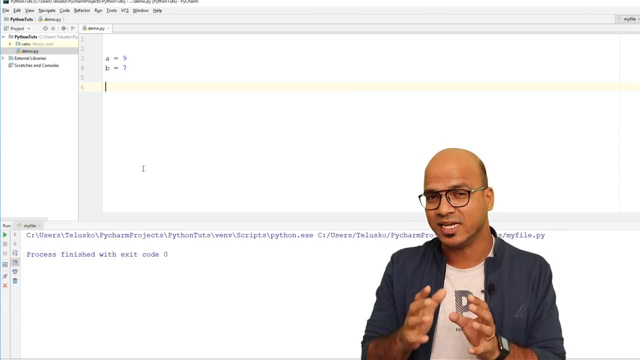 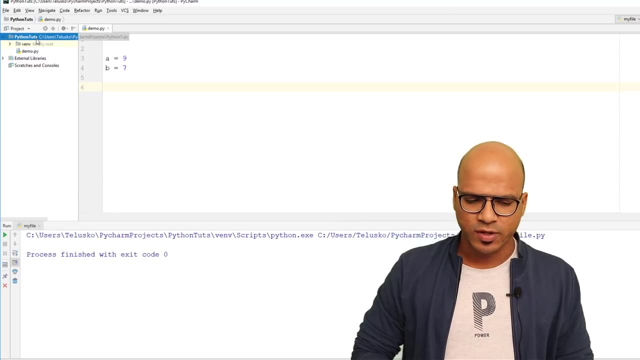 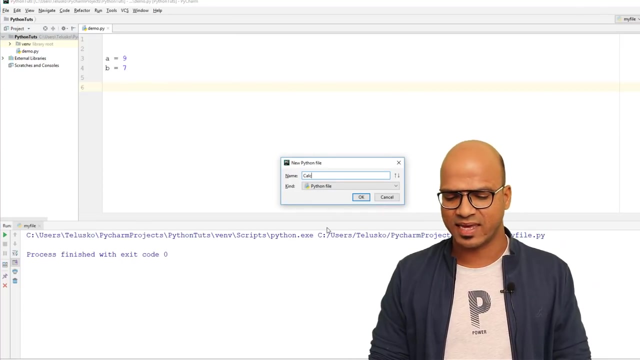 functions here in the same module, or you can create a separate module which will have all these functions and that makes more sense, right, having a separate module. so let's do that. so what i will do? i will create a new file, so i will say new and let's go to python file. we'll name this as a calc. 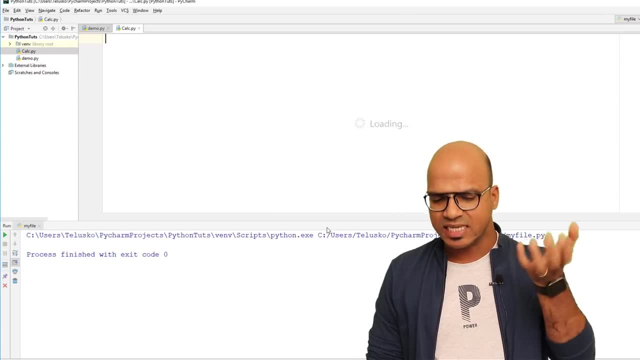 because this calc will have all the functions which you need. so this is a separate module for you. and let's define the function. so we'll say def and the function name would be add, which takes two parameters, which is a and b in this case, and we'll simply return a plus b. that's our first. 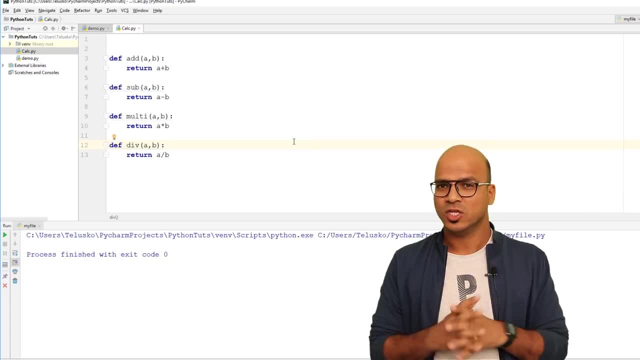 function. likewise, we can create four functions. let me do it quickly so you can see. now we have that here. now i want to use this function in another module, which is demo. how can i use that? so, because if i simply type add, it will not work right. you cannot simply call add it, of course it. 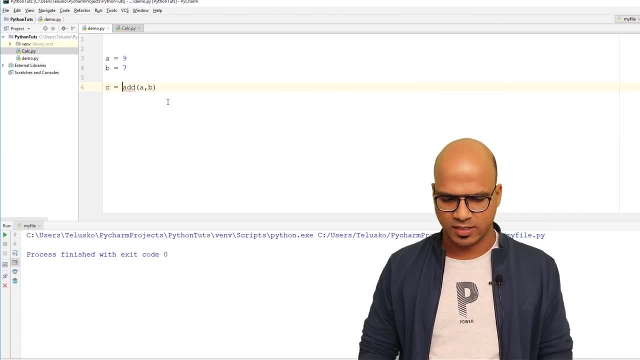 will not work directly. so even if i pass a comma b by saying a c equal to add a comma b, it will not work because it is in separate module. so we have used some inbuilt modules till this point, right. so, if you remember, we have worked with import, right. so we should say import something and then 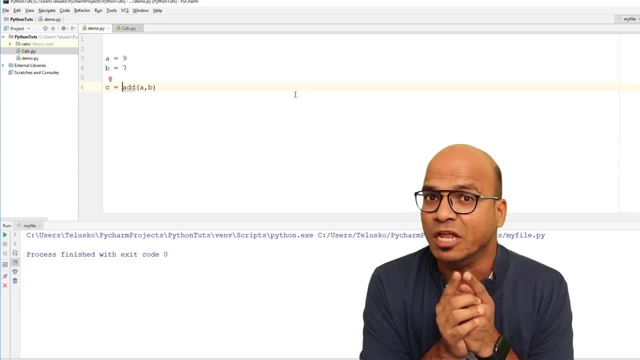 or the classes. we have done that right, but we have done that for the inbuilt modules. how about our own module? because calc is my own module now. so what i will do is, if you want to use calc, we need to import it, and the way you do that is by saying import calc. the job is done, you're saying import. 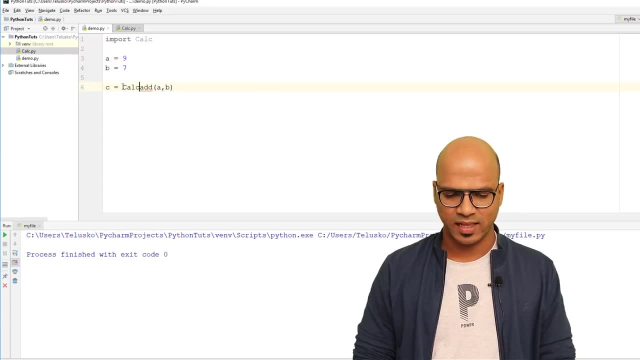 calc and whenever you want to use it, you will simply say calc, dot add. so this is one way, right, you can use a module name and then say dot add. or if you don't want to say calc every time, because of course, if you want to add, if you want to, 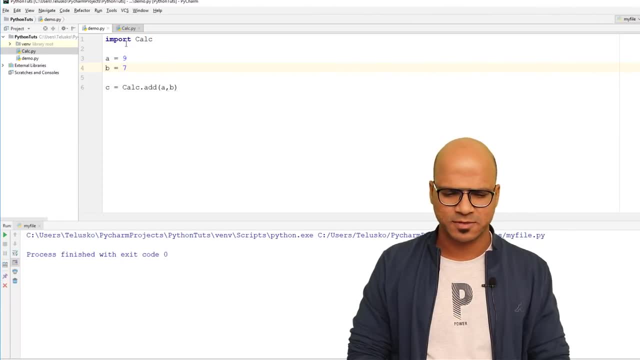 subtract, you will be using calcsubtract, calcmultiply, multiple times. instead of that, you can say from calc, import. whatever you want to import, i can say import, add. so in the one line you can say add. in the next line you can say import, sub, import, multi, or you can say import. 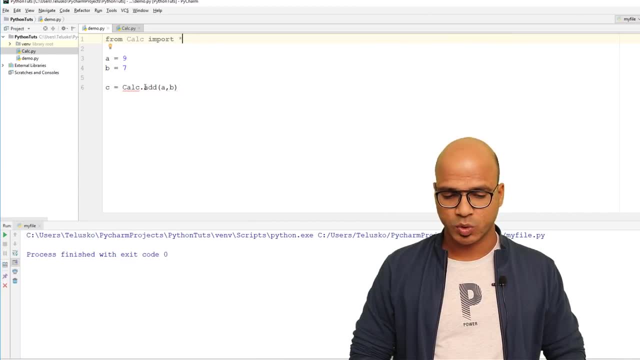 start right. it will import all the functions for you, and now you don't need to call calc. it will simply say add. it will work. right. it's a beauty, right? so this is how you break down your project into small, small parts, and of course, it doesn't make sense to have a separate module for separate 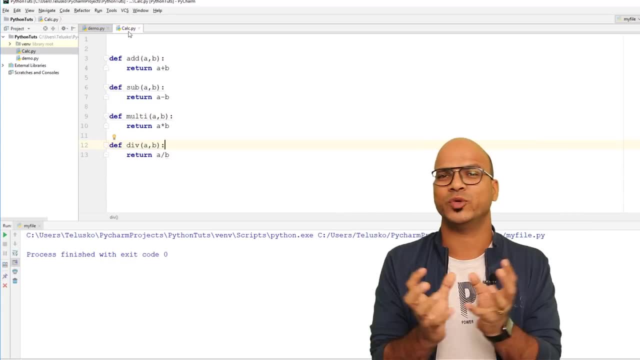 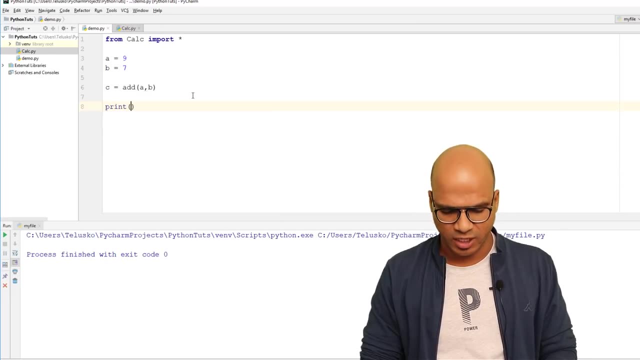 functions, right, so all your logical functions should work together in one module, not just function classes, variables, whatever you want, right. and now, once we got this, you can print the value of c and it perfectly works. let's run this. okay, so you can see. we got the output, which is 16: 1 and 6. 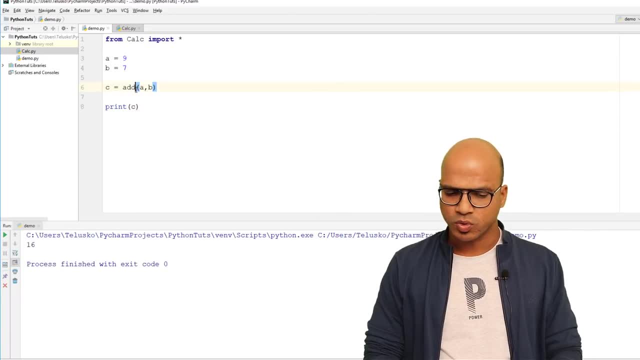 so that's what we wanted, right? 9 plus 7 is 16. we can also do that for subtraction. everything will work here and you can see we got two. so that's how you use modules. you can create multiple modules, not just one or two. you can create 10 different files as a different module.